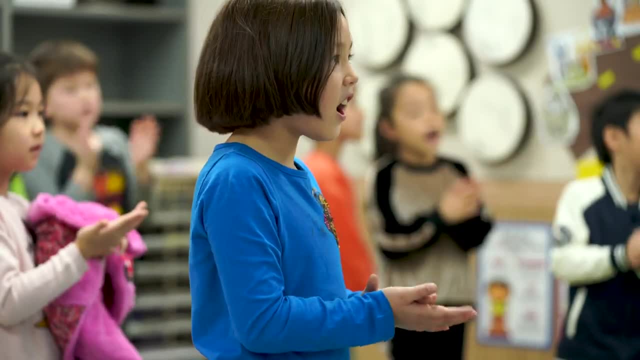 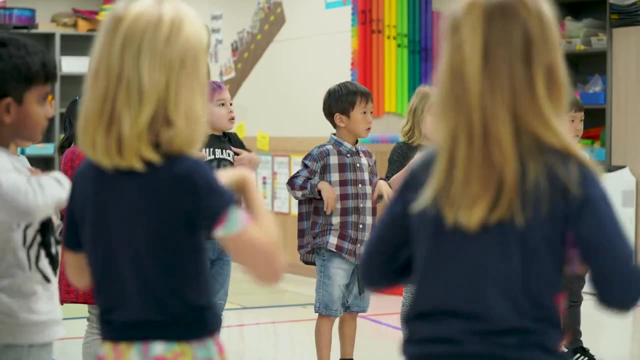 And our approach here at KIS, when we are teaching movement in music education, is to give them a movement vocabulary so that they can later on use the movements that they've learned through the music and to connect with those emotions that the music evokes and to use. 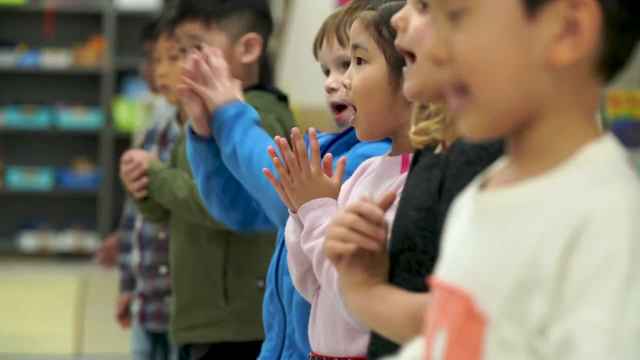 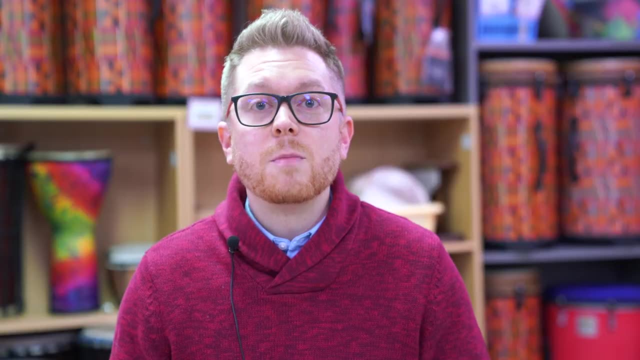 their body to express those emotions, Thank you. And then they can use their creative outlet to use their body to sort of be part of the song and to express their emotions through the music, through their body. Okay, Like this Through: yeah. 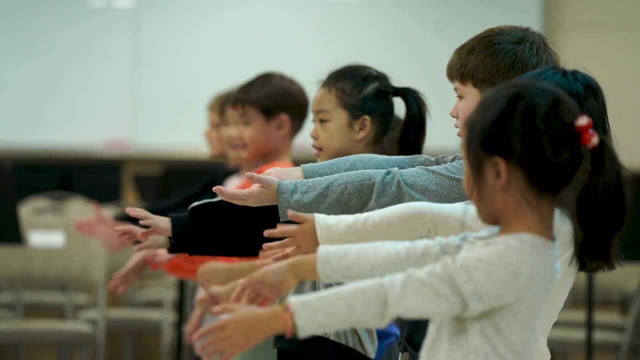 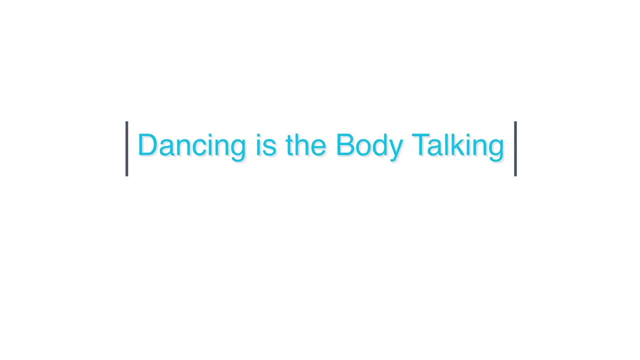 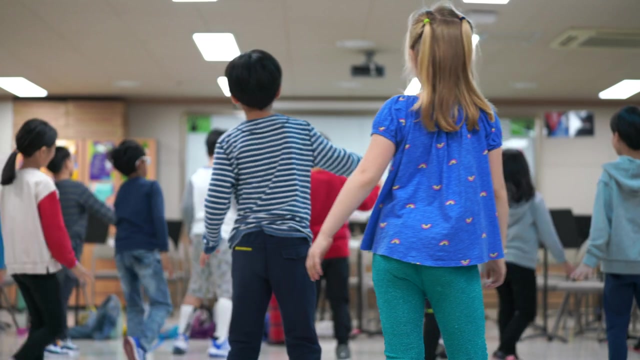 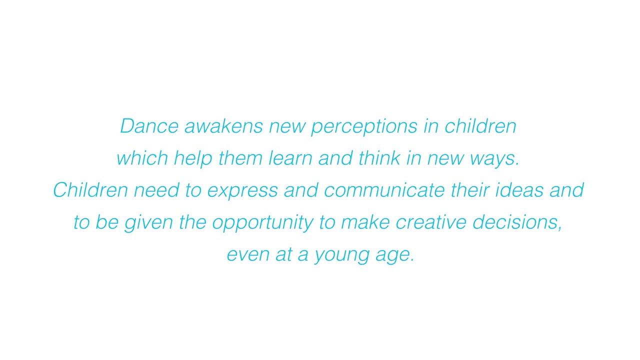 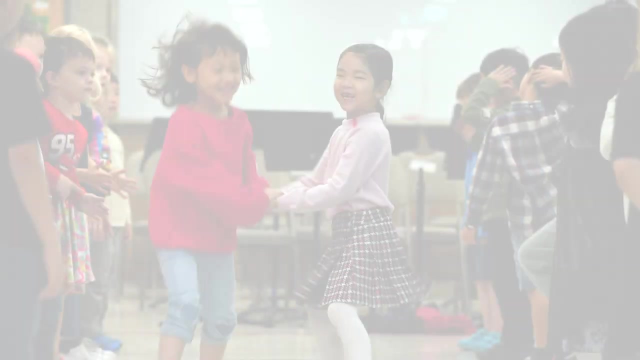 Through the alley. Baba handcолод, baba linga vague about babalinka. two hands round babalinka, two hands around babalinka. two hands Zing, Zing, Zing, Zing. 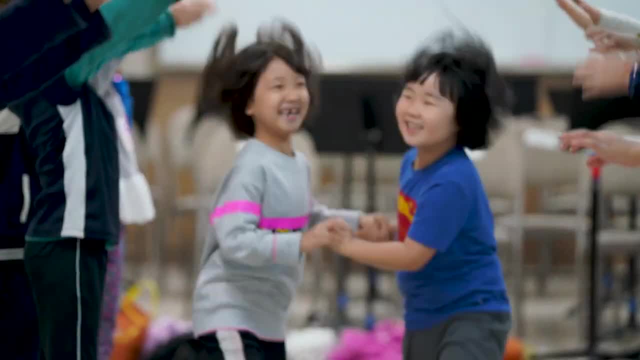 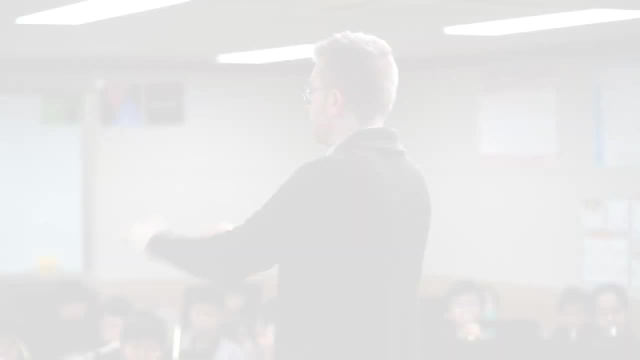 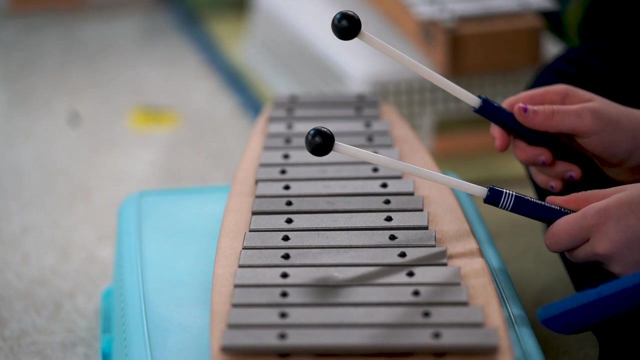